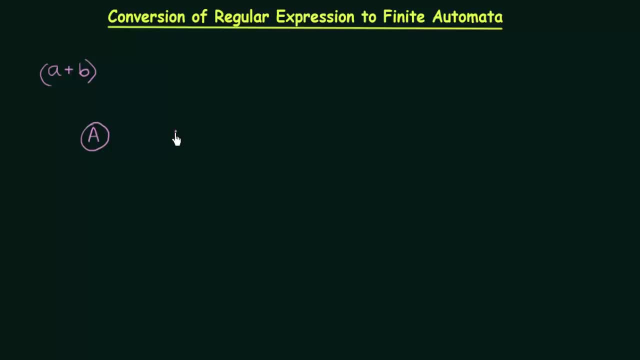 Let me call them states A and state B, And I can say that A will go to the next state B when it gets input small a, And also A on getting input small b. also it could go to the next state B. Or you could also express it in this way: 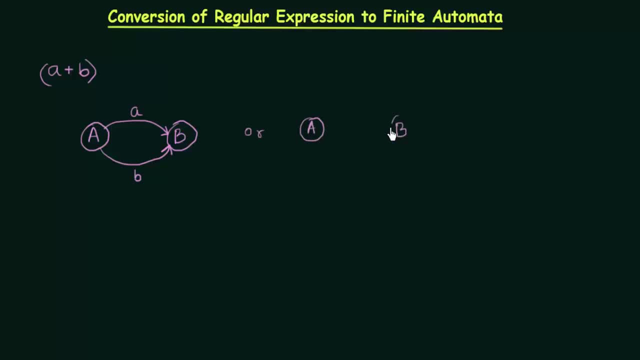 You can write A and B and instead of using two transition lines, just with one line you can represent, like this: A or B. So this means that A union B, That means A or B. So the state on getting either input A or input B. 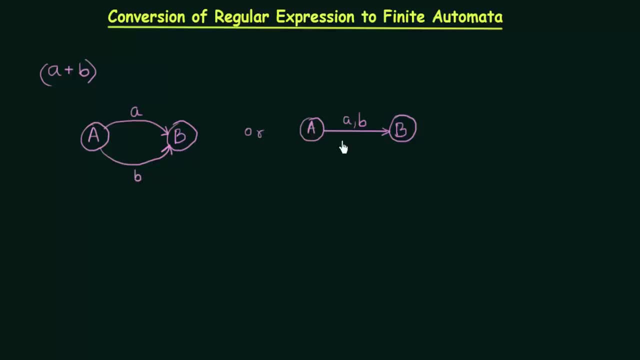 it can go to the next state, that is, B. So this is the same thing represented here, just using one transition line, A, on getting either input A or input B, It can go to the next state, B. So whenever you have a regular expression of this form, 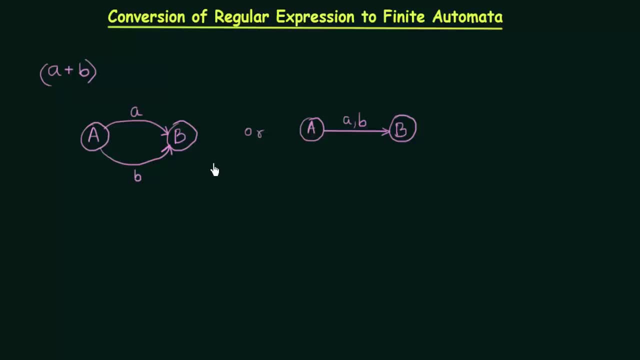 this is how you will design the finite automata for that. Alright, so let's see another expression. There is another expression that we were familiar in. our regular expressions were of this form: A, dot, B or just. it used to be sometimes represented as just A, B. 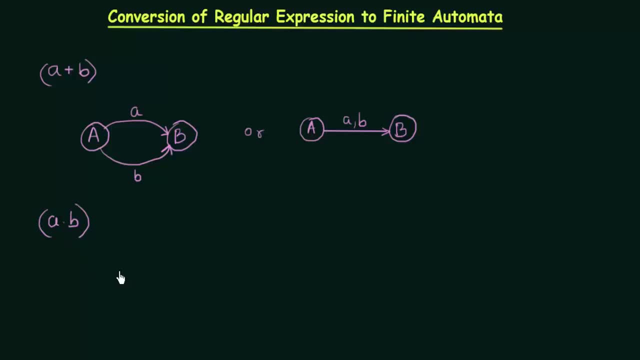 So when you have expressions of this form, you need to have three states: A, B and C, And we can say that A will go to the next state B on getting input small a, and B will go to the next state C on getting input small b. 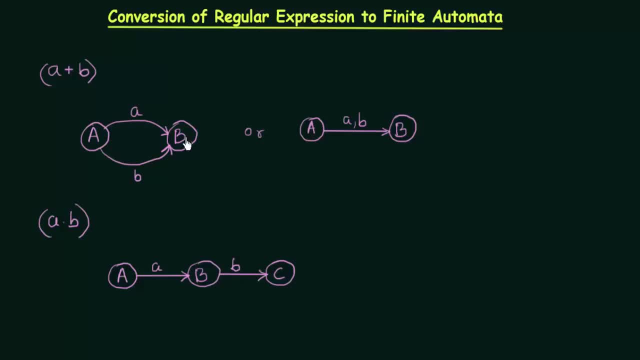 So here, unlike this, where it could go to the next state on either A or B, In this case it is not like that. In this case it will go to the next state on getting the function B first input a, and it will proceed to the next state again when it gets the next input b. so 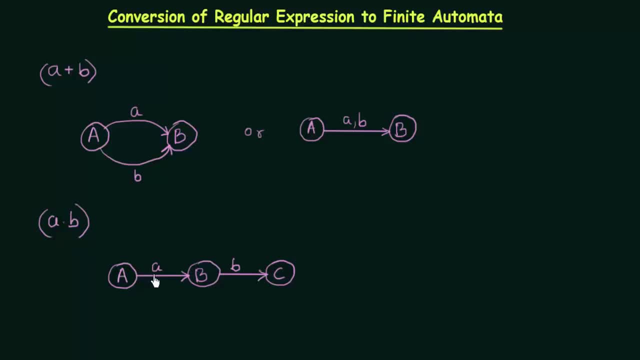 when you have expressions of the form a- b, you have to specify two different transitions for those inputs, a and b, unlike this one. all right, so this is how you do it when you have this kind of expression. okay, now we can see another expression that is a star closure of a, which we have already.